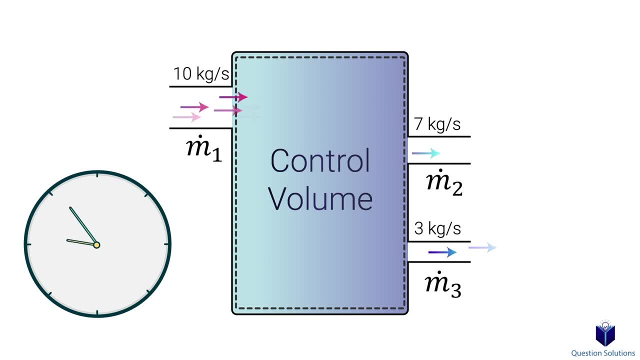 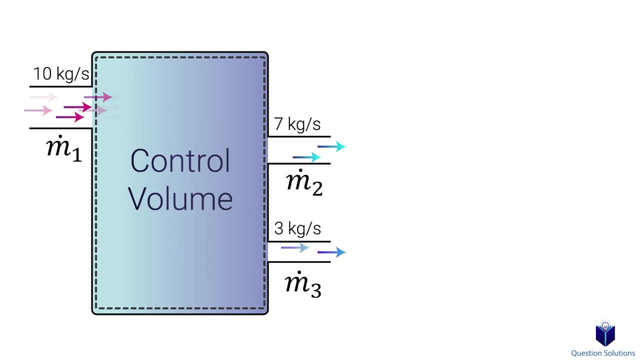 per second, the top one at 7 kilograms per second and the bottom one at 3 kilograms per second. Now, if we sum the mass flow coming in and then sum the mass flow leaving, then those two will be equal. We can represent that like this. So again, 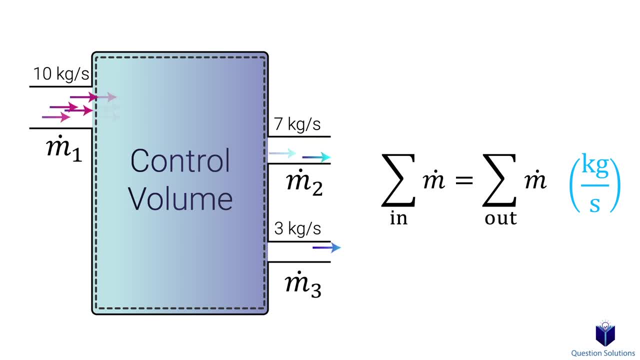 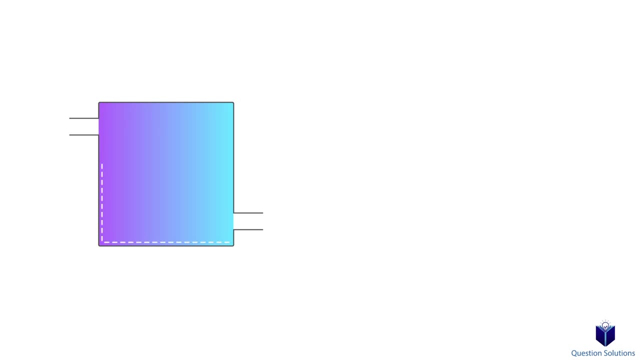 while individual inlets and outlets might have different mass flows, the total coming in must equal the total leaving, And each of these inlets and outlets will have a steady mass flow, meaning the rate of mass flow won't change with time. For a system that has a single stream, 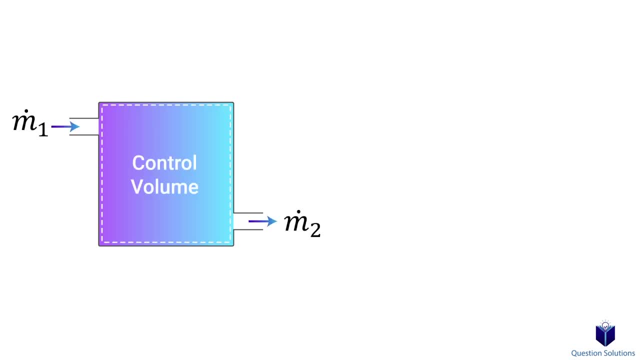 so that means one entrance and one exit. then we can write a mass balance equation like this: Each mass flow can be found by multiplying the density by the average velocity, by the cross-sectional area normal to the flow direction During a steady flow system. 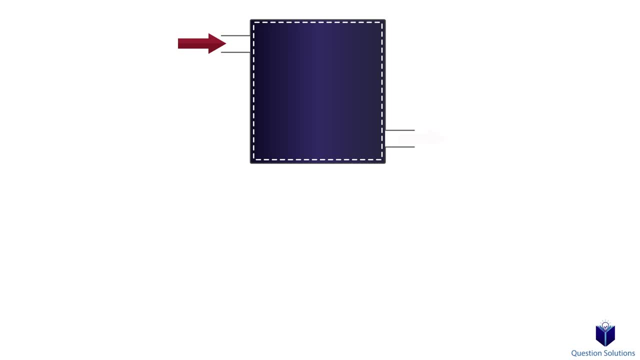 the amount of energy entering a control volume must equal the amount of energy leaving the system. We can write that like this. So this could be heat work or mass. We can expand this equation to cover all the types of energy we just mentioned. Remember from the previous video that this theta. 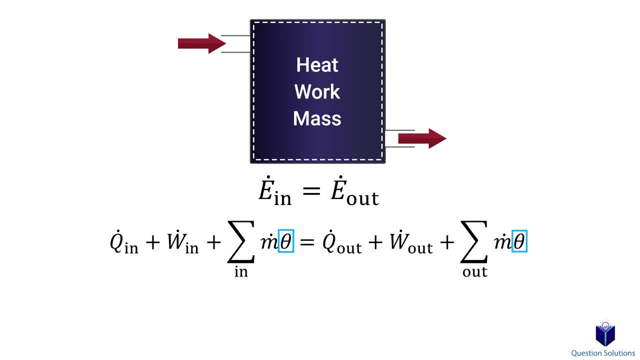 symbol represents the energy of a flowing fluid, So we can expand it further like this. Let's go through each term. This is the rate of heat transfer between the system and the surroundings. This is power. This is mass flow. This is enthalpy. This is the kinetic energy. 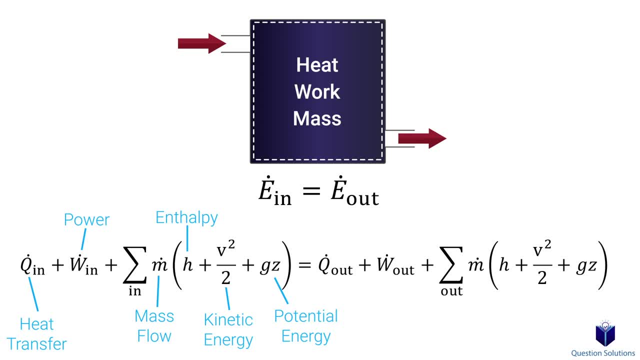 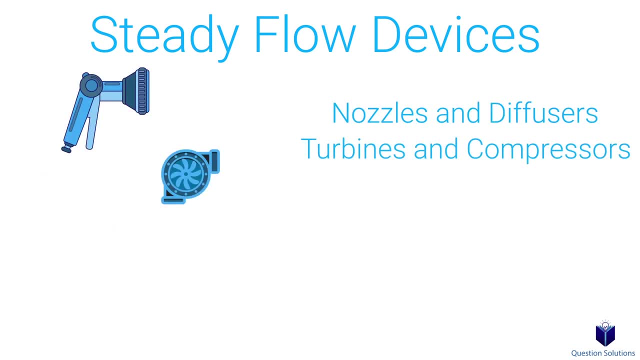 And this is potential energy. There are a lot of different types of steady flow devices. Some of them include nozzles and diffusers, turbines and compressors, throttling valves, mixing chambers, heat exchangers and pipes and ducts. In this video, we're looking at just nozzles. 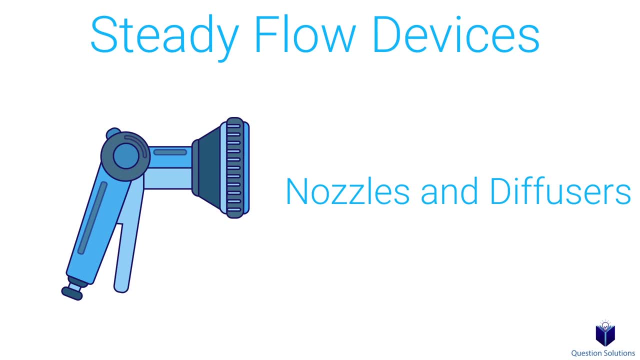 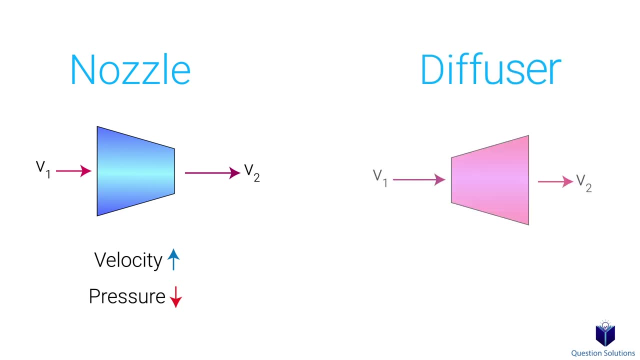 and diffusers, And in the future videos we will cover the rest. A nozzle is a device that increases the velocity of a fluid by reducing the pressure. A diffuser, on the other hand, increases pressure by reducing the velocity of the fluid. You probably experienced this. 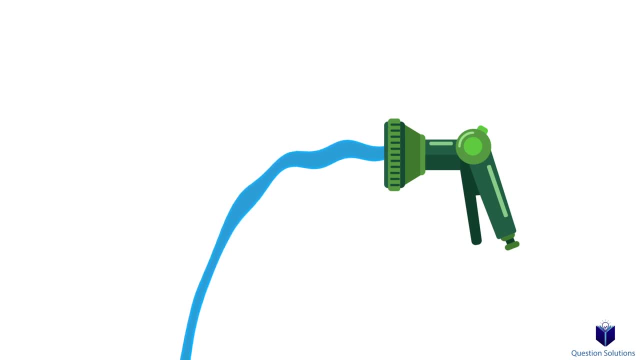 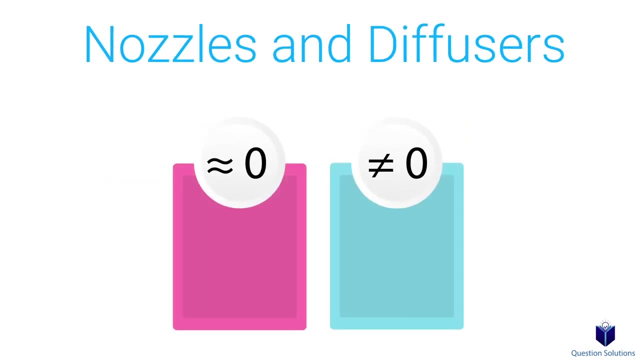 with garden hose nozzles, But nozzles and diffusers are also in jet engines, rockets and more. There are some general characteristics for nozzles and diffusers that you should keep in mind. Usually, the rate of heat transfer between the fluid that's flowing through the system. 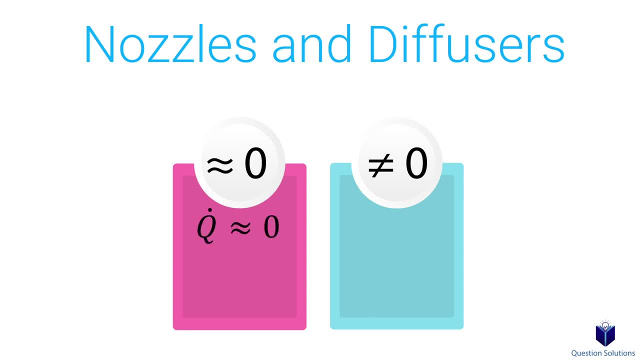 with the surroundings is small, So small that it's negligible, Which means Q dot is usually zero. The work involved when it comes to nozzles and diffusers are also negligible. Also, change in potential energy is negligible. However, the fluid in nozzles and diffusers tend to experience large 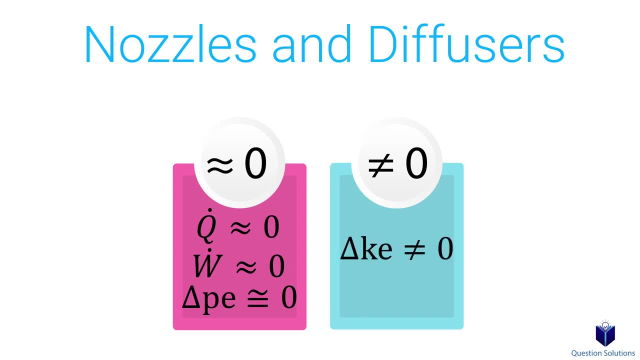 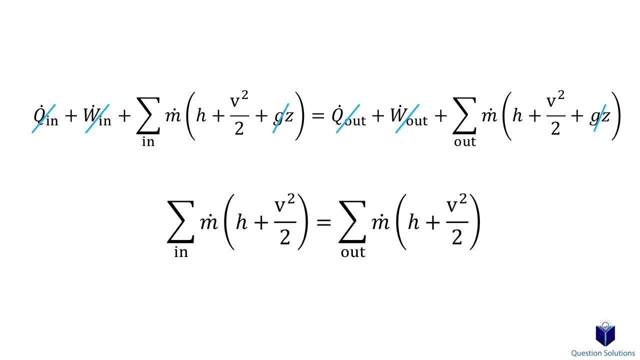 velocity, So kinetic energy will not be zero. Keeping this in mind, our big energy balance equation will usually simplify to look like this: So we have enthalpy change and velocity change. Remember that enthalpy change can be found by using this equation, So we multiply specific. 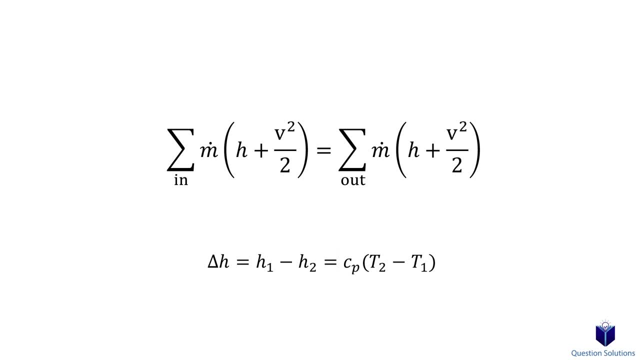 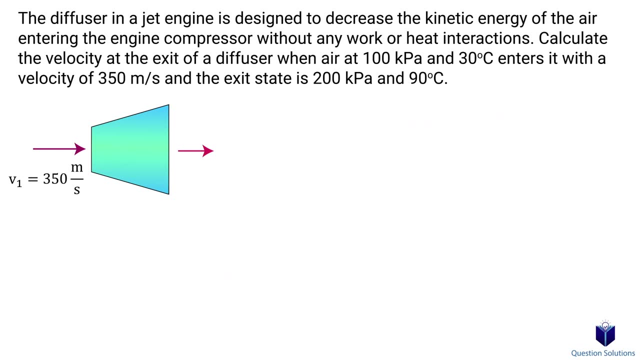 heat by the change in temperature. Keeping all of this in mind, let's go through some examples to see how we can apply what we learned In this question. we have a jet engine that decreases the kinetic energy of the air entering the compressor. We need to figure out the velocity. 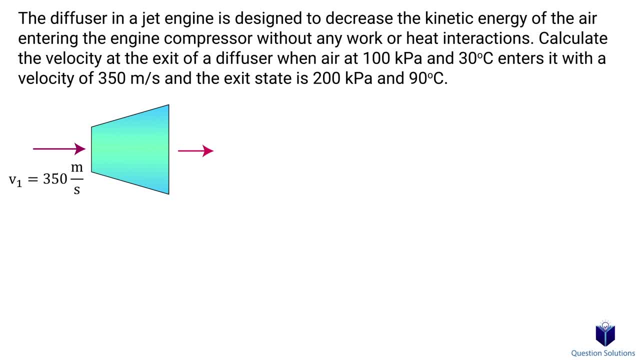 of the air as it exits the diffuser. Let's write down what we know. The initial pressure is 100 kilopascals and initial temperature is 30 degrees celsius. The air enters at a velocity of 350 meters per second. At the exit side, the pressure is 200 kilopascals and the temperature is 90. 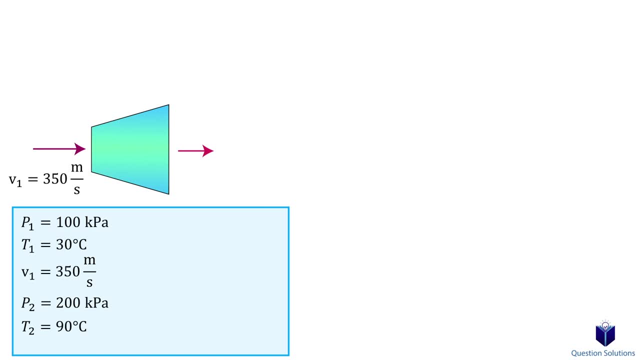 degrees celsius. We will start off by writing down our energy balance equation for a standard flow process. So rate of energy in is equal to the rate of energy out. We can express all of the energy that's associated with the system like this. Now, since this is a diffuser problem, 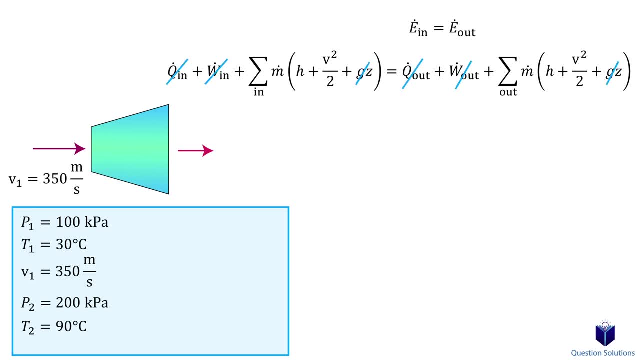 there is no work, heat transfer is negligible and potential energy change is also negligible. That means we just need to consider enthalpy and kinetic energy. so our equation simplifies to this. The mass flow is the same, since it's one inlet and one exit, so we can cancel. 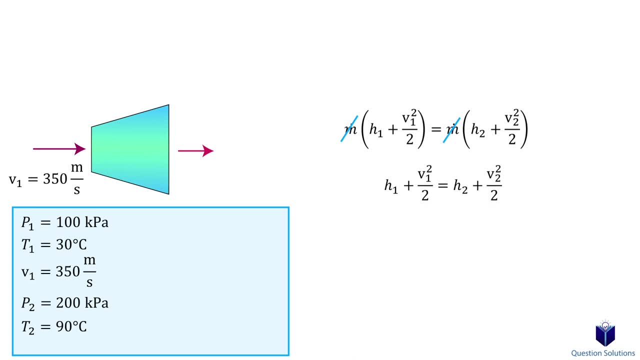 them out. to further simplify our equation, We can bring enthalpy to one side and kinetic energy to the other side. Enthalpy can be found using this equation, so we can replace it. Next, multiply everything by 2 to get rid of the fractions. We have everything we need, except 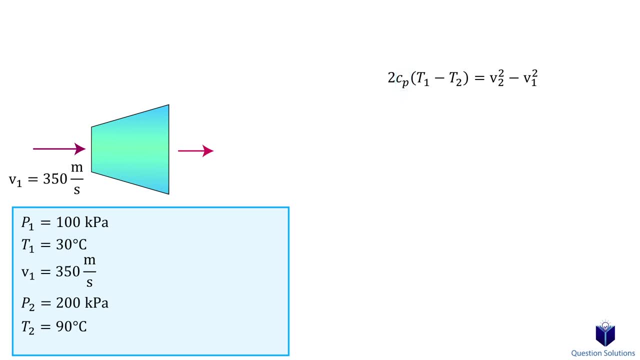 for the specific heat value. To find it we can use a table, but we need the average temperature to use it. So we just add up the initial and final temperature and divide it by 2. We get 60 degrees celsius. 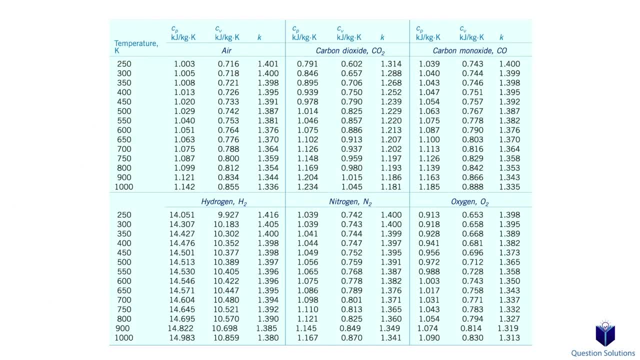 or 333 kelvin. Now we can look at our table. So at 333 kelvin, our value would be between 1.005 and 1.008.. So we will extrapolate and use 1.007.. Now we can go back to our equation. 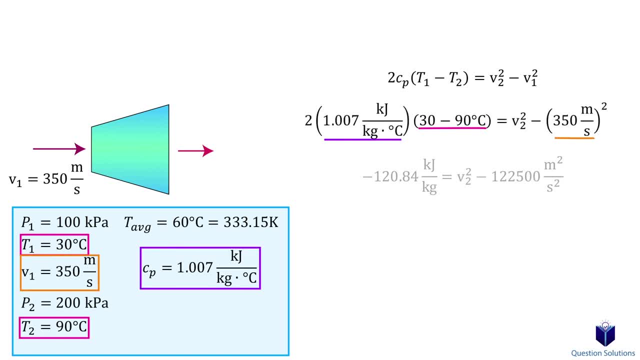 and start plugging in values. When we simplify, we get square meters over seconds squared, which is equal to joules per kilogram. Problem is our left side value is in kilojoules per kilogram, So we need to multiply it by 1000 to get it in joules per kilogram. Now we can take the square. 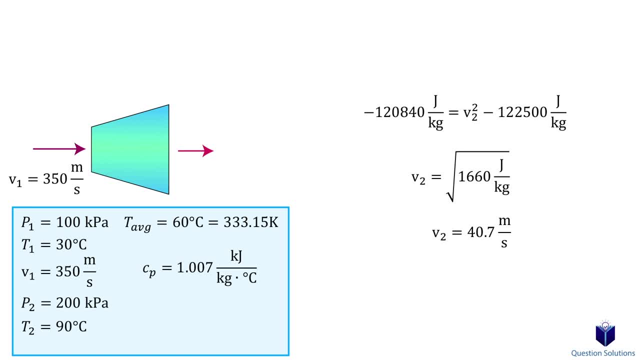 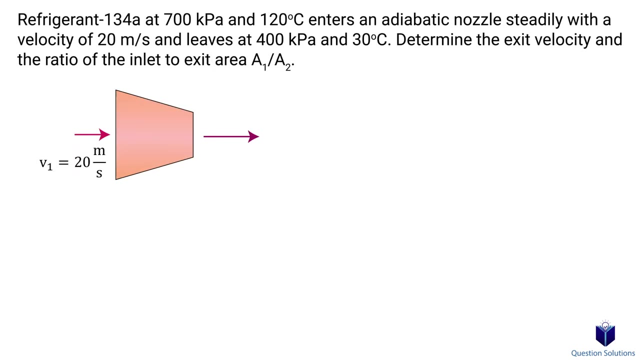 root and that gives us 40.7 meters per second. Remember again that joules per kilogram is equal to meters squared over seconds squared. so taking the square root gives us meters per second. Let's take a look at this problem where we have refrigerant 134a. 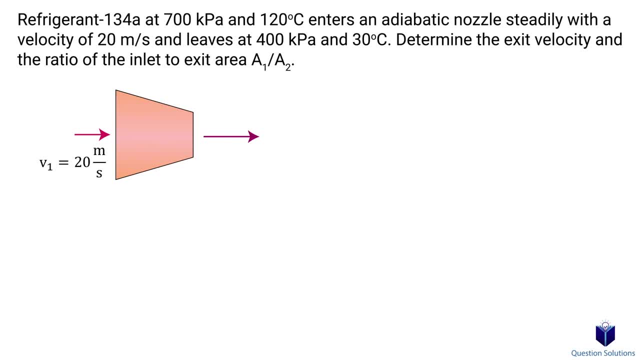 entering a nozzle and we need to figure out the exit velocity and the ratio of the inlet to the exit area. First we will write down what we know. The initial pressure is 700 kilopascals, the initial temperature is 120 degrees celsius and the initial velocity is 20 meters per second. 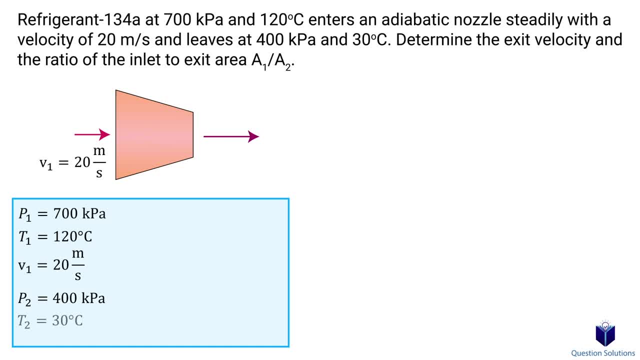 The final pressure is 400 kilopascals and the temperature is 30 degrees celsius. So, as usual, we start off with our energy balance equation, Since this is a nozzle. our work is zero, heat transfer is negligible and potential energy change is also negligible. 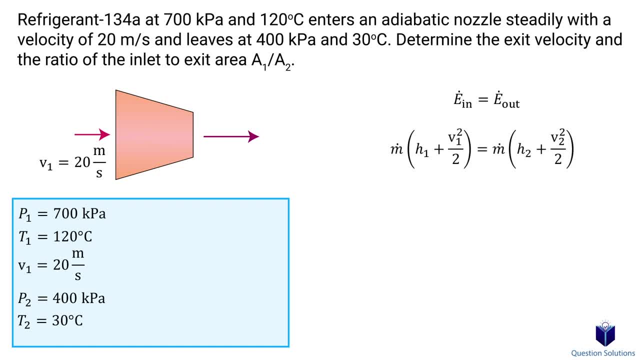 We need to consider enthalpy and kinetic energy. Since in the nozzle we have one inlet and one outlet, the mass flow is the same, so we can cancel it out. Since this is R134a, we can actually figure out the enthalpy values. 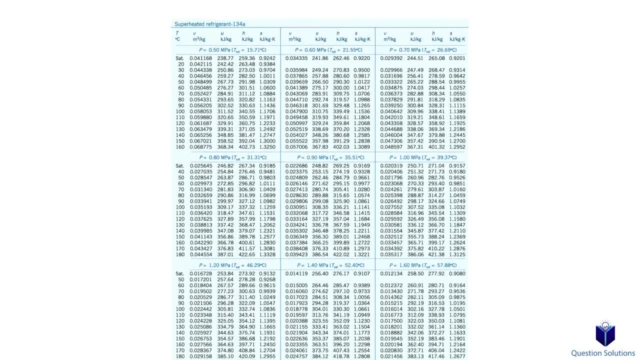 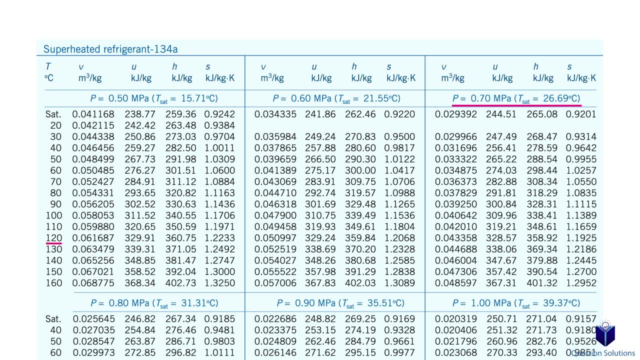 based on the given information by looking them up on the superheated refrigerant table For initial enthalpy the pressure is 700 kilopascals and the temperature is 120 degrees celsius. So the value we are looking for is right here. For the initial pressure, we have 700 kilopascals. 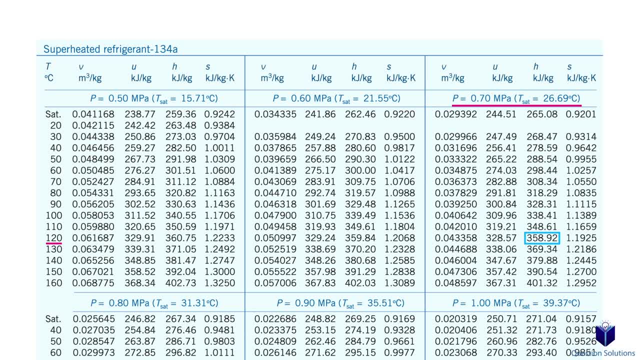 and the temperature is 120 degrees celsius. So the value we are looking for is right here. For the next part of our question, we will need the specific volume, so I'm going to write that down, since we have the table up. That's the value right here For final enthalpy. 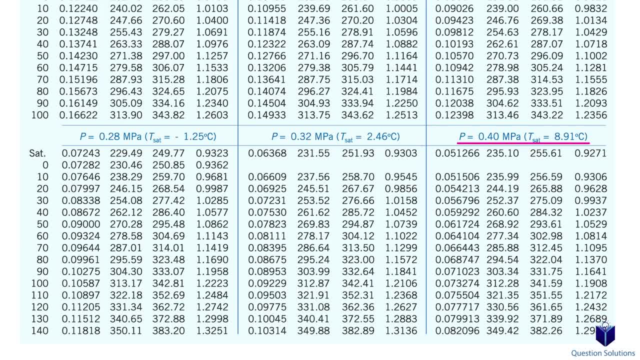 the pressure is 400 kilopascals and the temperature is 30 degrees celsius, So the value we need is right here. Again, I'm going to write down the specific volume value as well. Now that we have these values, we can plug them into our equation. 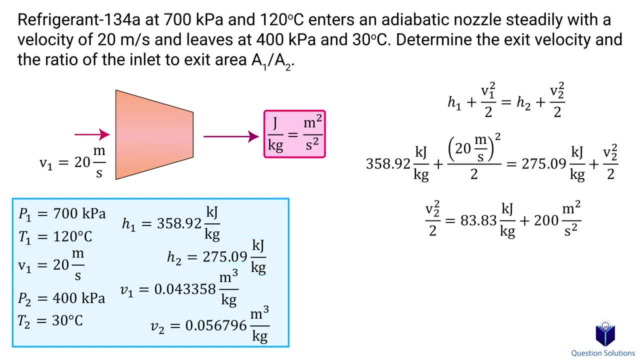 Remember that square meters over seconds squared is joules per kilogram, so we need to multiply the kilojoules value by 1000 to make sure our units are the same. Solving by taking the square root gives us 409.9 meters per second. 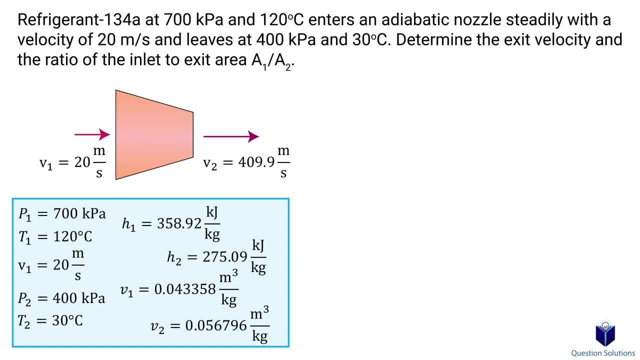 The next part of the question asks us to calculate the ratio of the inlet to the exit area of the nozzle. For that we just need to use the mass balance equation. We can expand further by writing down the equation for mass flow. Then we need to eliminate density, since we don't have that value. 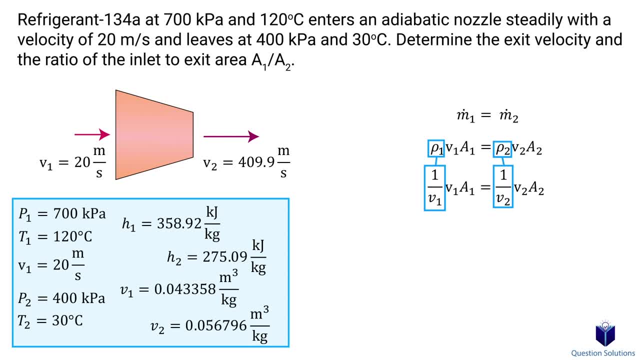 Remember that density is 1 over specific volume, so let's replace it Now. we will isolate this equation so that we have a ratio of a1 over a2.. Don't get the specific volume and velocity confused, even though the letters look similar. So now we can plug our values in, because remember 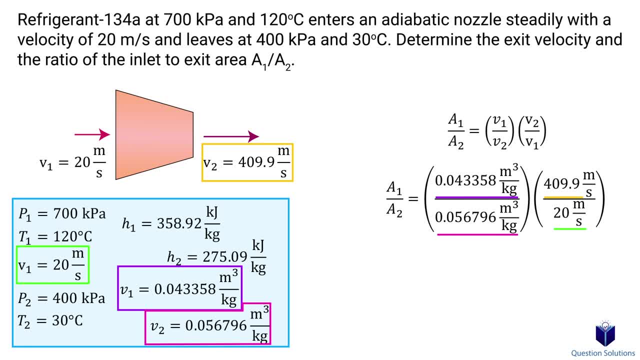 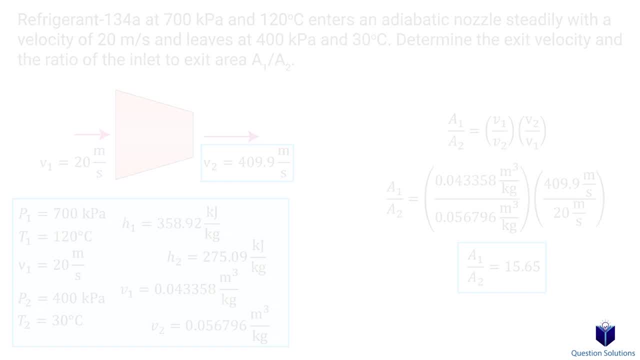 we found the specific volume values before. Don't forget that we found the final velocity in the previous step of the question. Let's solve and we get our ratio In this question. we have steam entering a nozzle and we need to figure out the mass flow rate. 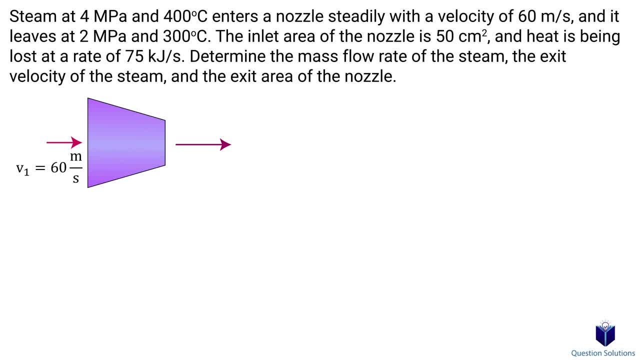 the exit velocity of the steam and the exit area. Let's start off by writing down what we know. The initial pressure is 4 MPa, the temperature is 400 degrees Celsius and the velocity is 60 meters per second. When the steam exits, it leaves with a pressure of 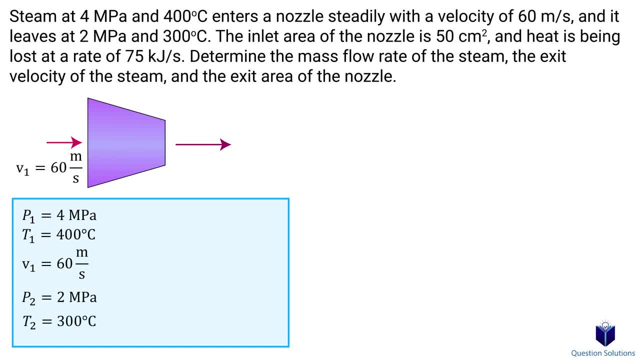 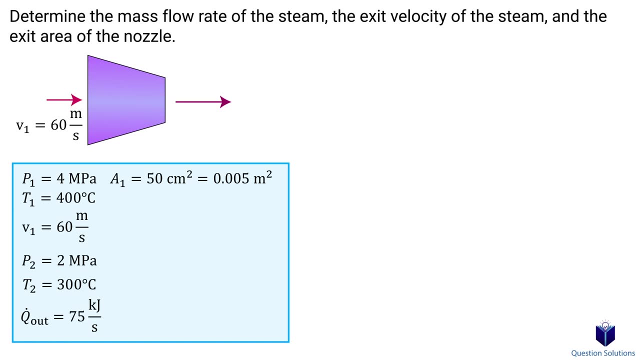 2 MPa and the temperature is 300 degrees Celsius. The inlet area of the nozzle is 50 square centimeters and we're told that there is a heat loss of 75 kJ per second. For this problem, we're going to need specific volume values and enthalpy values. So let's 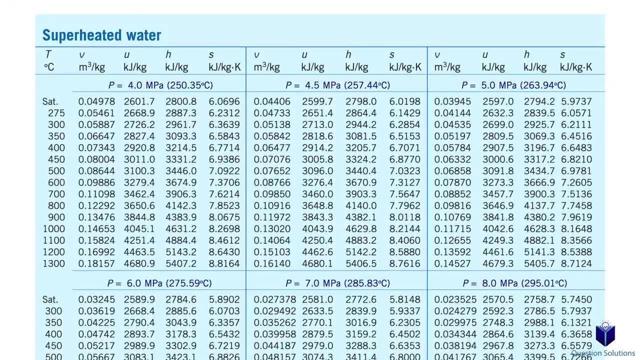 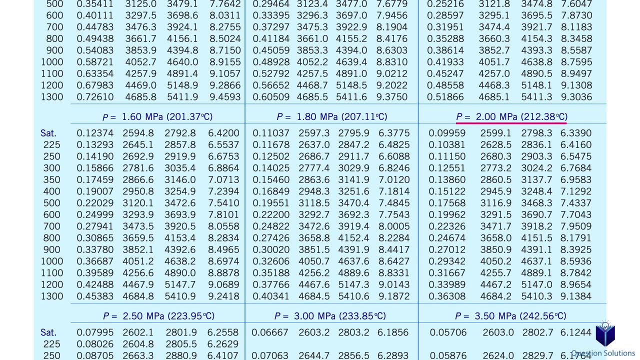 figure those out using steam tables. The initial pressure is 4 MPa and the temperature is 400 degrees Celsius, so our specific volume value is right here and our enthalpy value is here. Next we have a pressure of 2 MPa and a temperature of 300 degrees Celsius.